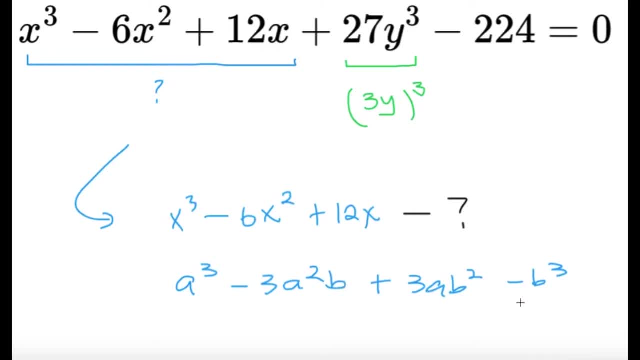 and then it kind of motivates me to try if b equals 2.. Now, indeed, if you try b equals 2, if b was equal to 2, based from like a nice guess- again, I just kind of guessed, based from the terms here- but if you try b equals 2, you're really gonna- oops, you're really gonna. 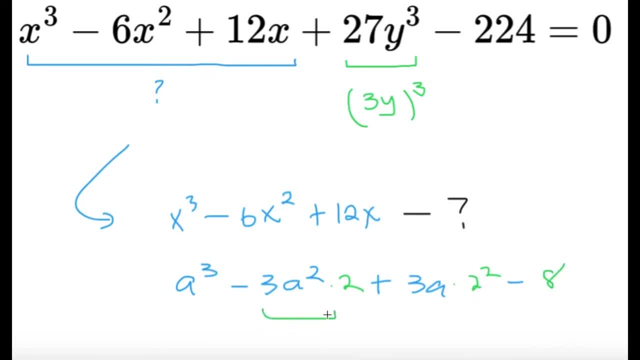 get a cubed minus. well, this becomes like minus 6a squared, this becomes like positive 12a and the minus 8, so I guess we can kind of make the nice conclusion that, indeed, I guess we can kind of complete the cube here just by doing a minus 8, and that's going to be the. 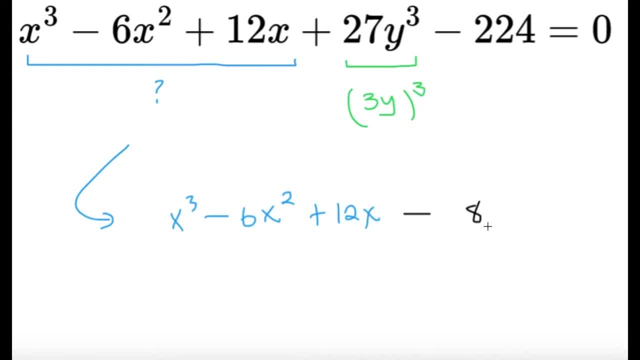 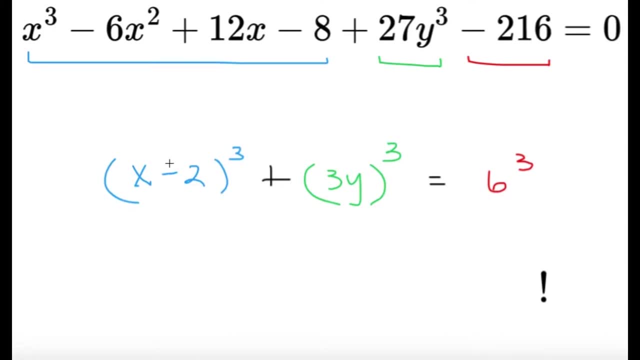 because maybe there will be something nice, because it is something in terms of like sum of cubes. maybe that's the intended solution to the question. All right, so now that we observe that it is kind of related, let's try to complete the cube here: x cubed minus 6x, squared plus 12x. 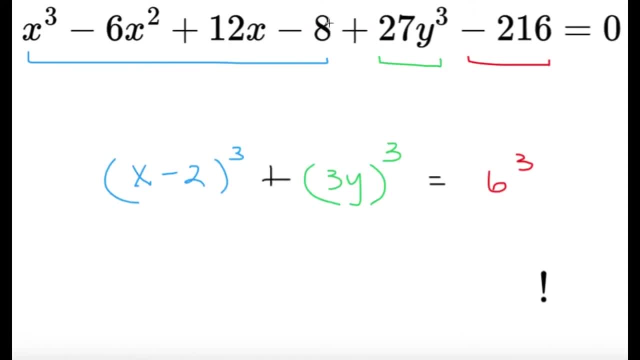 minus 8, so I just extracted- whoops, I just extracted a minus 8 from this. minus 2,, 2, 4, and then leaving us with minus 216 here Now, 216, that's an oddly familiar number. it's actually. 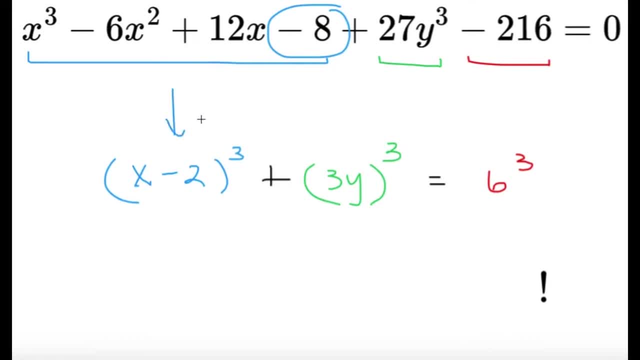 So what I did here is what I'm going to make: this x minus 2 cubed, so completing the cube. we have another cube here from the 21,, a 27y cube, and then we're going to put this negative 216 on. 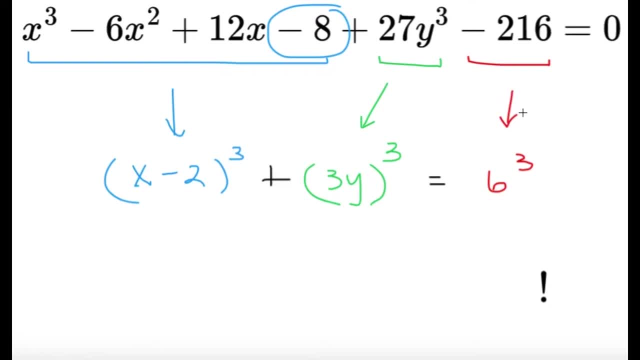 the other side and then that's going to be equal to 6 cubed. All right. so, as intended from the question, we have a sum of cubes equal to another cube scenario, All right. it's not very often that we see a lot of sum of cubes equal to the cube. 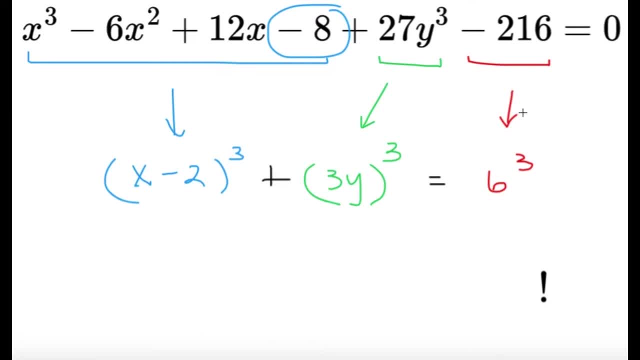 So here's another integer scenario and we kind of recall a nice theorem on sum of powers. So this kind of looks like the format a cubed plus b cubed equals c cubed, which is something related to this, and it's actually the Fermat's last theorem. Now it's kind of weird that we're. 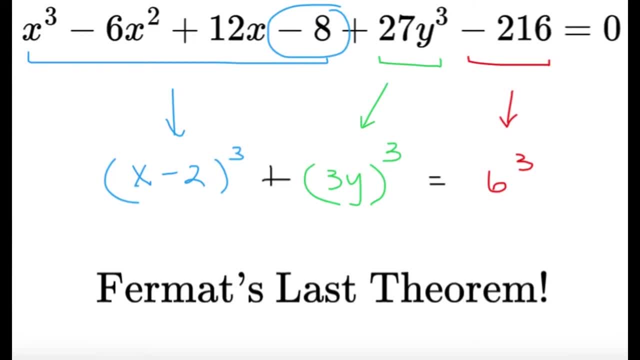 using the Fermat's last theorem, because the Fermat's last theorem tells us about having no solutions. but all right, we don't have, we have, we don't. we should never do that. forget, like the statement of the Fermat's Last Theorem, and that is that. 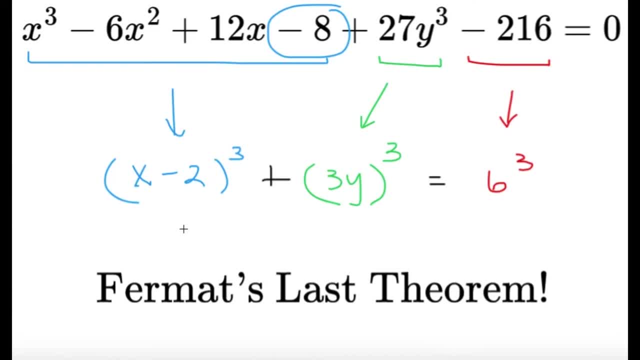 tells us that there are no positive integer triples- a, b, c- to the solution. a cube plus b cube equals c cube. so that's the rule: there are no positive integer solution. I guess it kind of makes sense. if B was 0, then a could equal C, right, or? 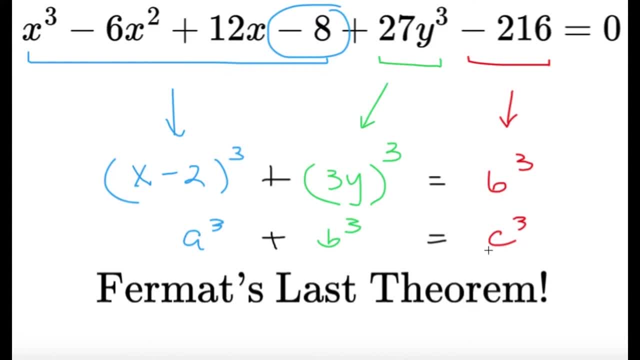 like a, B could equal to negative a, and then C would be 0. so I guess it is nice for us to remember. oh yeah, we shouldn't forget the description or the statement of the theorem. now there are no positive integer triples, so I think there would. 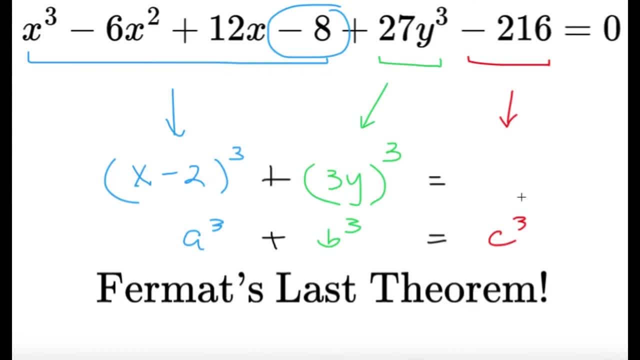 be no solutions, if I mean, since 6 here is already positive, so we don't really have to do worry about that. but we just have to consider the 3y not being positive and then the X minus 2 not being positive to find all the possible. 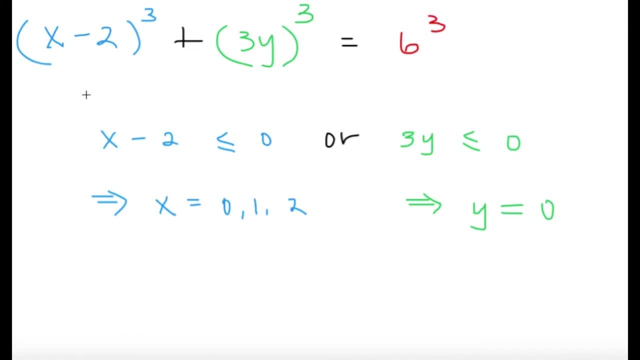 solutions. so what we have to do is just the following: because we know that by Fermat's Last Theorem these two cannot be both positive. so these two cannot be both positive. so I guess we should just take cases here. so we should just have at least one of these two being less than or equal to 0. 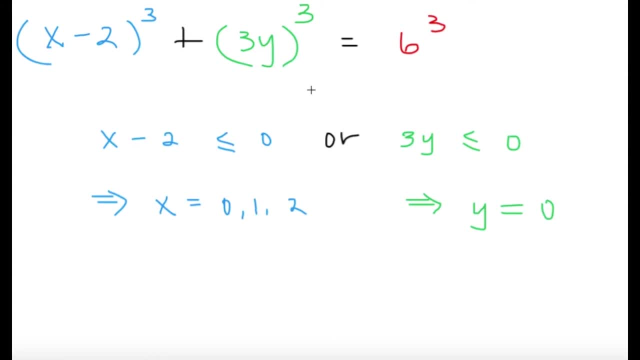 so we just have X minus 2 less than or equal to 0 or the 3y less than or equal to 0. now we have a restriction for X and Y, which was X and Y must be non-negative integers. so we just have to solve for X and Y. 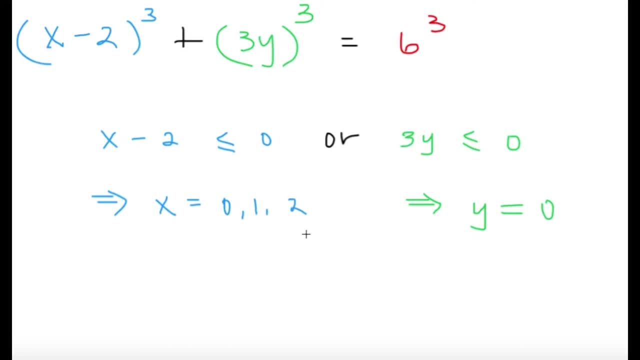 respectively. so X is equal to 0, 1 or 0, 1 and 2. Y is equal to 0. again, it's an or scenario, so we have to check for all four of these and to see if we get like a value or like a pair of solutions for the question. alright, so after using the 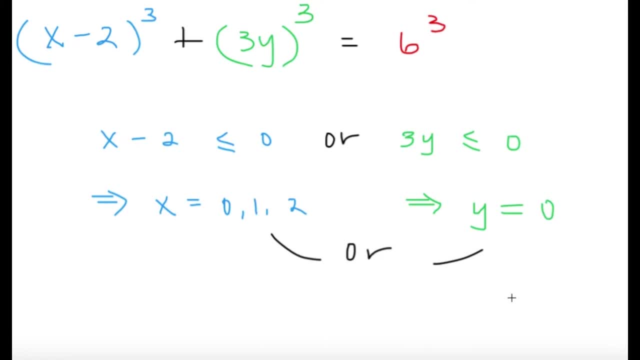 Fermat's Last Theorem. it's just checking finitely many cases, which is pretty nice, alright, so let's try the y equals 0 case. now, if y equals 0, we'll just imagine this not being here anymore. so X minus 2 cubed it's gonna. 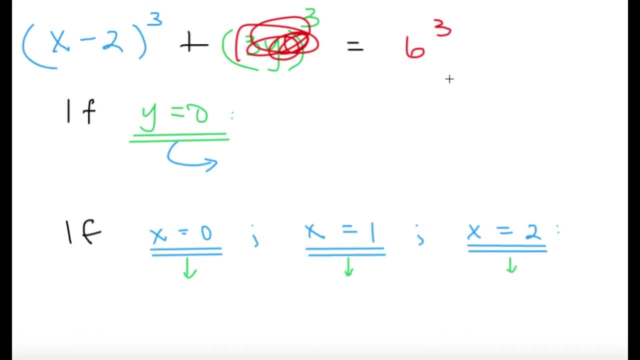 give us 6 cubes. I think it's pretty obvious for us to say X minus 2 would equal 6 and that's gonna give us X equals 8. alright, so apparently 8: 0 is a solution. and let's try to check if X equals 0. oh, actually, if X equals 0 and X, 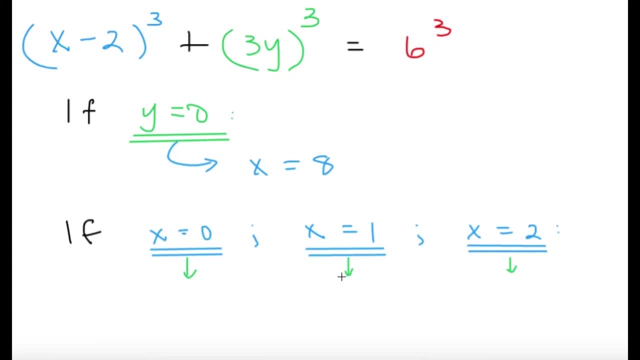 equals 1. I'm pretty sure that there are no solutions now. why is that the case? because, well, we have a multiple of 3 here. it is 3 y cubed. so this is a multiple of three, well, 6 cube. well, 6 is divisible by. 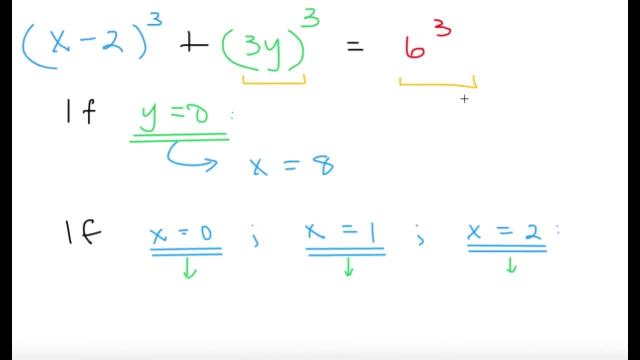 3. so 6 cube is obviously divisible by 3 you. so you can just use the kind of mod 3 or just a multiple of 3 idea and to say that I'm pretty sure this X minus 2 cube must also be a multiple of 3. but if X is 0 in X equals 1. take a look at this: X. 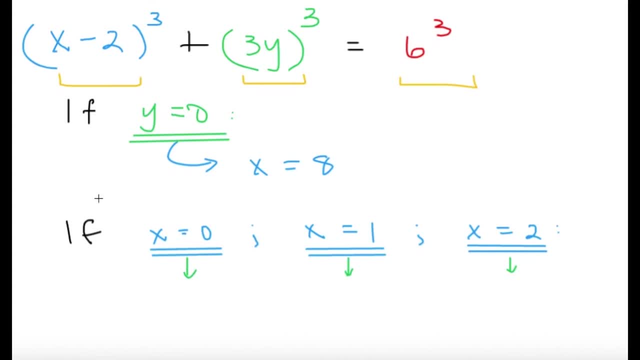 minus 2 cube term. if X equals 0, the X minus 2 cube, it's gonna become negative 8, the negative 2, so obviously not a multiple of 3. so I'm pretty sure there wouldn't be any solutions here. just because it is it doesn't satisfy or doesn't, it's not going to allow that kind of things, kind of. 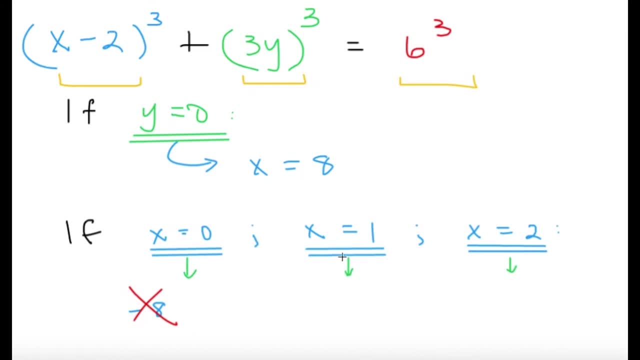 solutions under mod 3. technically checking the multiples of 3- and same can be said for x- equals 1, because if I substitute 1 in this x minus 2 cubed, that's going to be negative 1 cubed, so that's going to give us obviously negative 1. again same reasoning: it's not divisible by 3, so I don't. 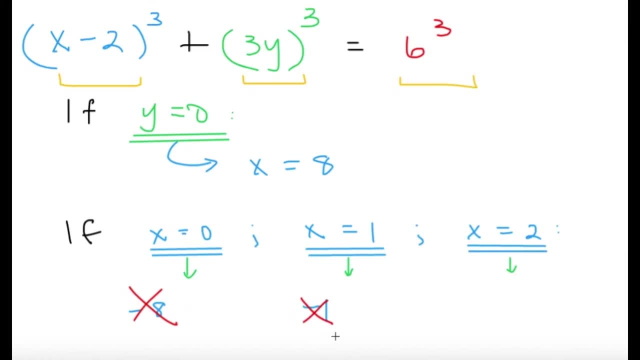 think we're going to we're able to get a solution just because everything fails just by taking a look at mod 3. so all right. last thing to check is: x equals 2, and I think that's pretty similar to the y equals 0 case, because if x equals 2, it's just this being gone, so we can just kind of 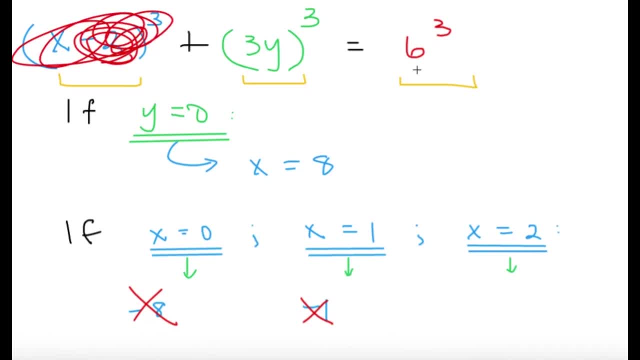 solve for y. so 3y must equal 6 then. so y would have to be equal to 2, because 3y equals 6, so y equals 2. so all right, apparently, just by checking these four values which are which are the only possible values of y and x, so we have two pairs. so apparently we're.